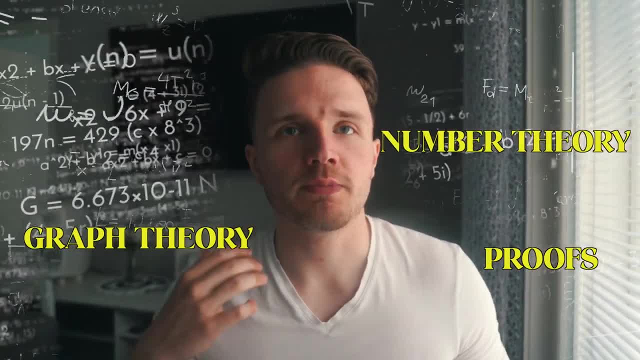 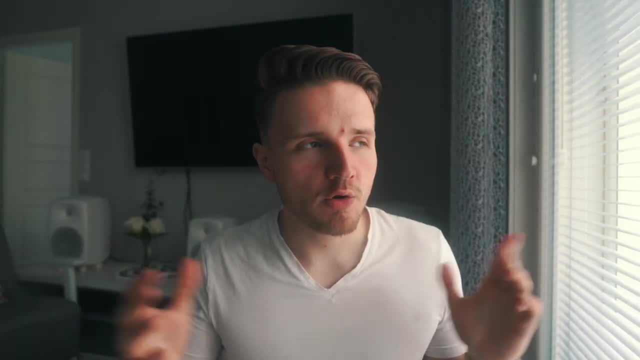 If you want to learn all the mathematics that you would ever need to know for computer science, this is probably the course for you, But I think the bigger question is that: should you learn the maths at all? Hello, and welcome back. In this video we are going to be reviewing the Mathematics for 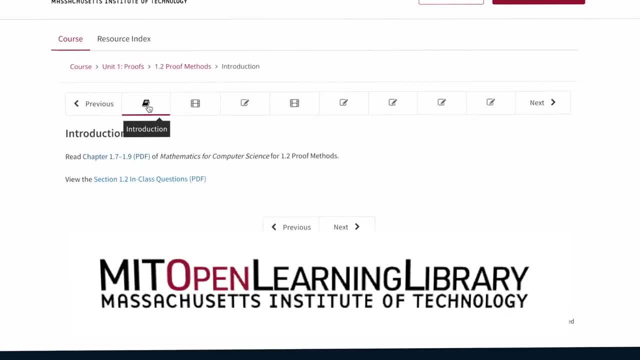 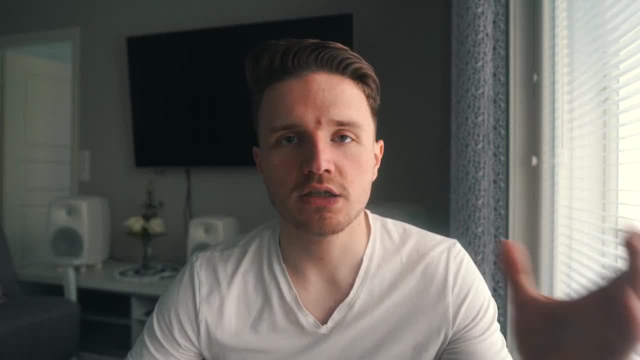 Computer Science free online open source course by the Massachusetts Institute of Technology Online Learning. This is the course that I personally did in the beginning of my journey of self-teaching computer science, and the purpose of this course is, as it states, to teach all the 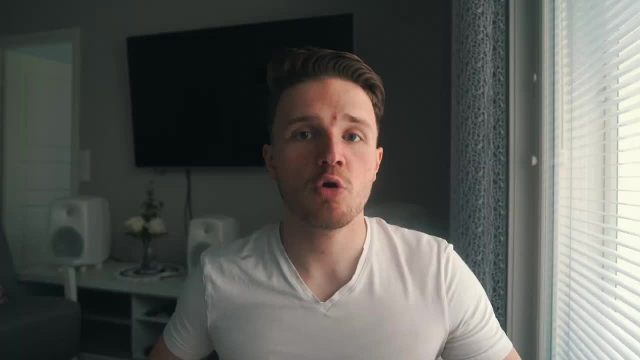 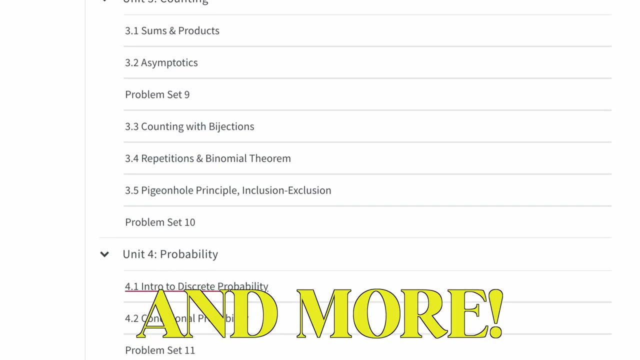 maths that you need to know for computer science. specifically, It'll go over topics like mathematical proofs, state machines, binary relations, graph theory, probability and a lot more- Basically, all the mathematics that is used in computer science. I'm going to be reviewing. 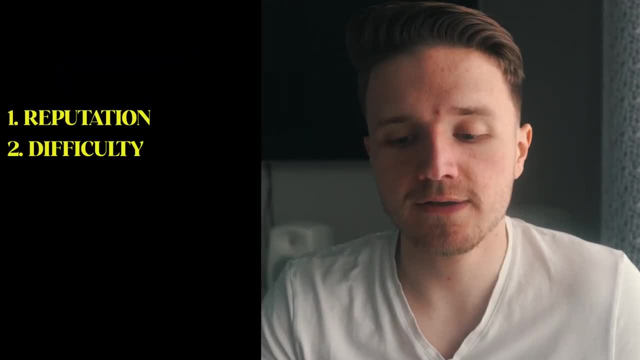 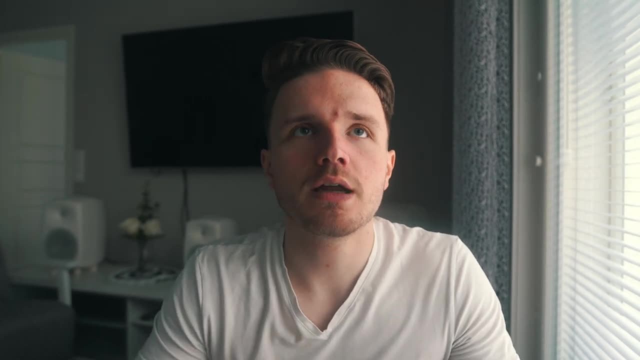 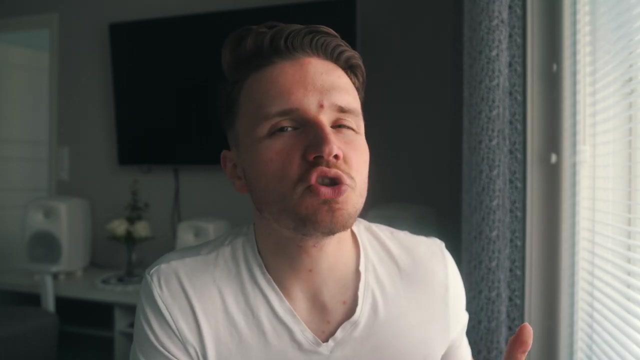 this course using the following criteria: reputation, difficulty, quality of instruction, cost, as well as comprehensiveness. But make sure to watch in the end, because I think there are specific types of people who should definitely take this course and there are also different kinds of people who probably shouldn't take this course. But let's get started with the. 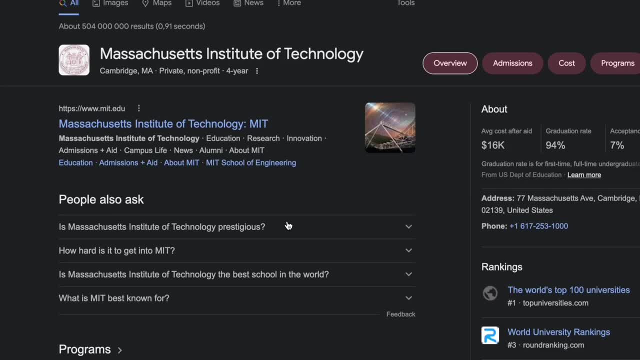 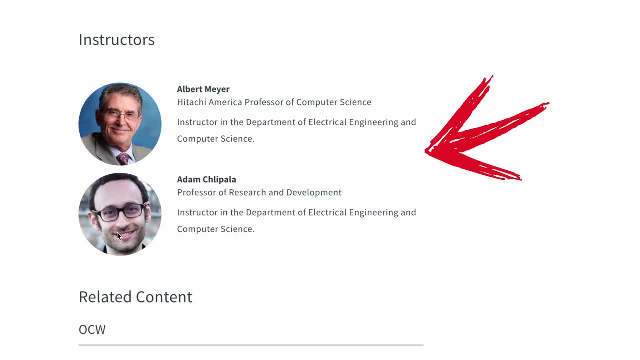 review In terms of reputation. well, it's by the Massachusetts Institute of Technology, which is a really renowned university. The lecturers and the people who have made this course are extremely renowned in the area of computer science. So I would say the reputation of this course is. 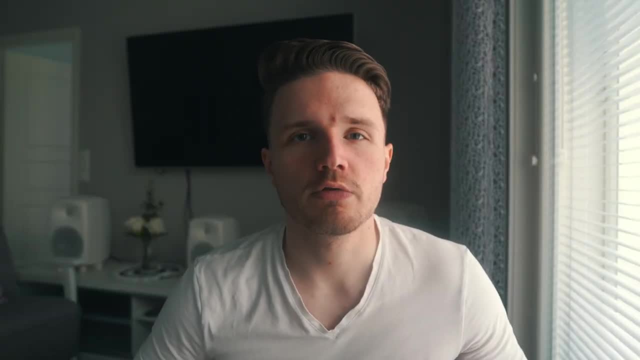 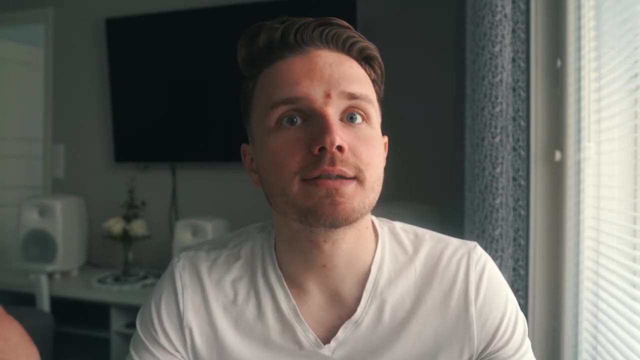 obviously extremely good. But so what are my thoughts on this course then? Well, first of all, in terms of difficulty, it is a very theoretical maths course, Which I mean? it is a maths course, and maths is, by definition, theoretical, And it is a rigorous course as well. It's not like 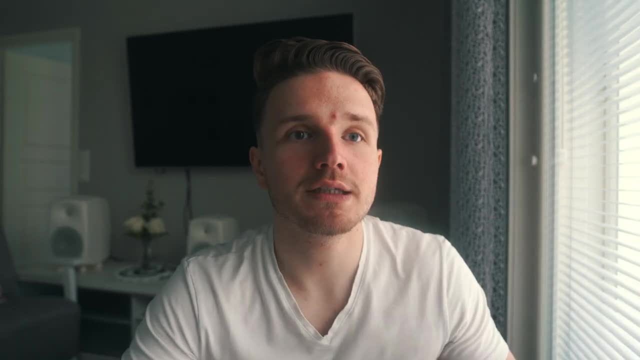 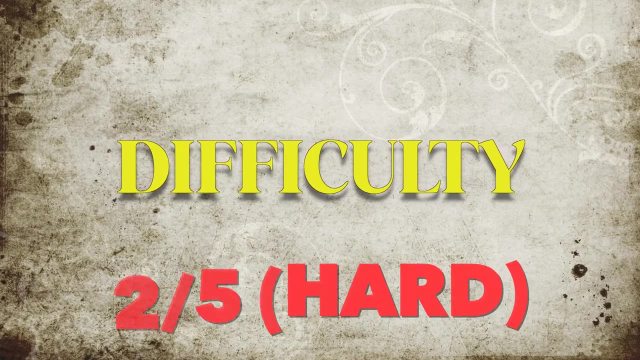 necessarily meant to just teach you like some high level ideas. No, it is a very rigorous math course that teaches maths in a very mathsy rigorous way. But even beyond that, I think it's structured really well in the sense that the problems will challenge you. 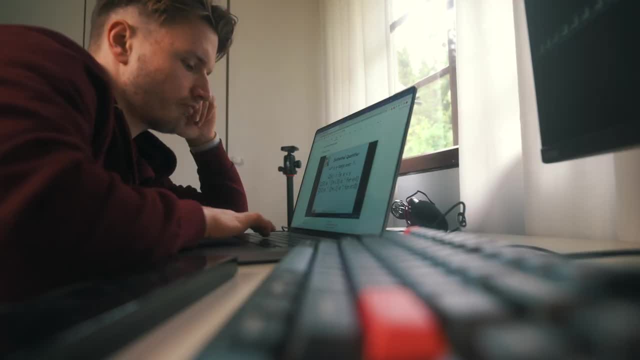 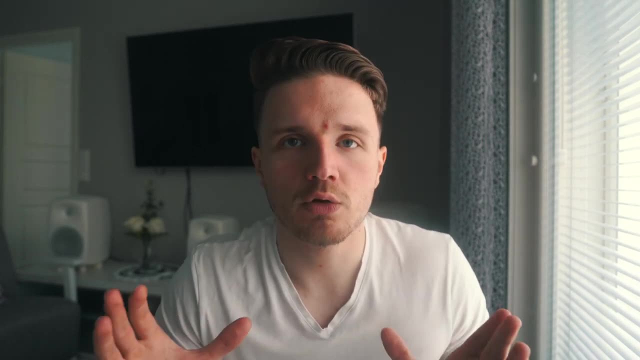 You won't be able to solve the problems by just copying something that you found on the textbook or from the lectures. They are actually going to challenge you to think and apply the things that you're learning, Which I think is the number one requirement that every good course should have. 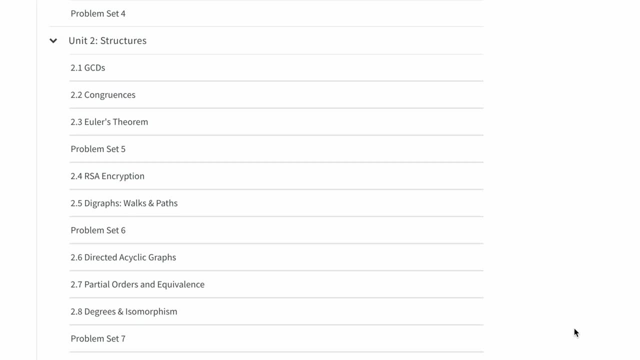 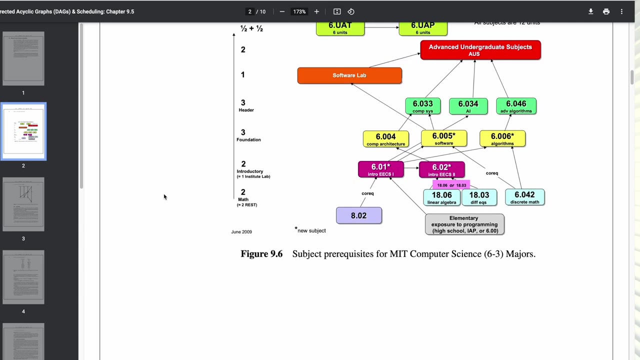 In terms of the structure of the course itself, it's divided into four sections and each of them have first lecture videos that go over the topics of that section, and then you also have an accompanying textbook- slash lecture notes that you will be using along the way And online the course. 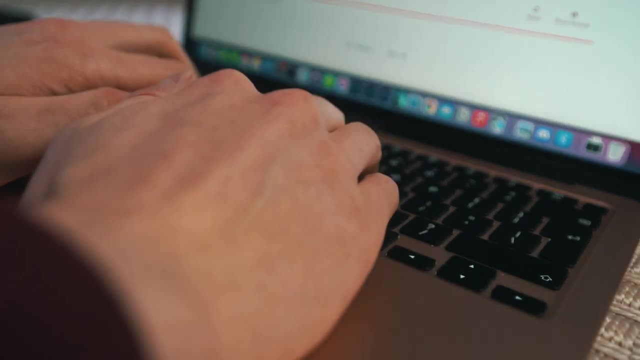 itself has quizzes to test your knowledge, but the textbook itself has a lot more problems as well for you to really drill down and really make sure you understand what you're learning. The only real challenge with this course is that it's very difficult to understand the text that you're learning. 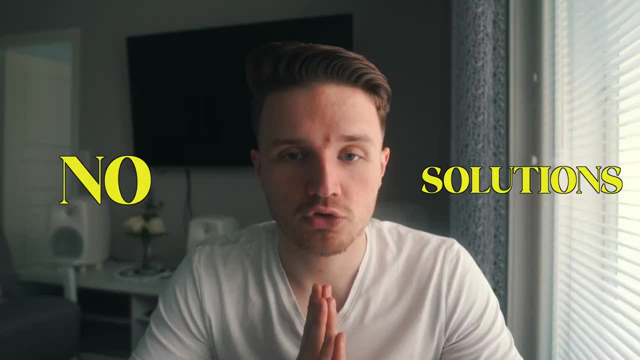 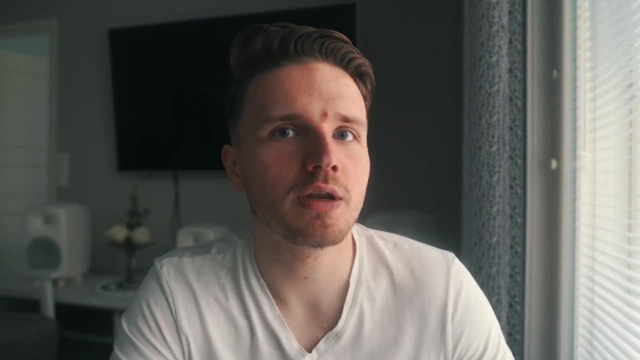 downside with the problems is that it doesn't have solutions, and this seems to be the case with so many of like math courses- is that they don't like to provide solutions to students because there's some there's really this belief on, like the math lecturer community, that there's no such thing as a 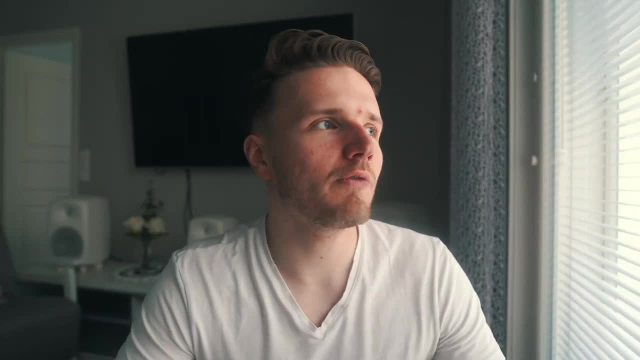 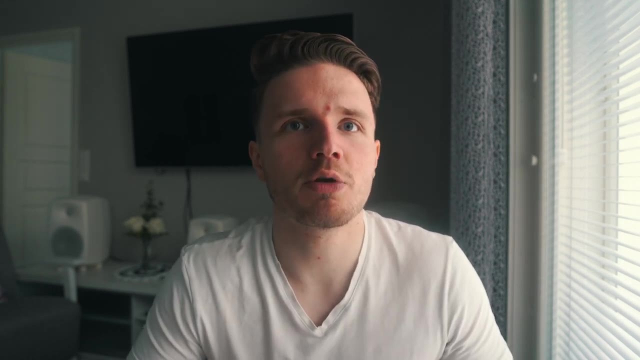 model solution, you need to find your own solution, blah, blah, blah like. it's not very helpful when you don't provide any sort of even answers to like. so just so that we know that we've done it right. essentially, i had the same problems with my mathematics for economics course i did part of 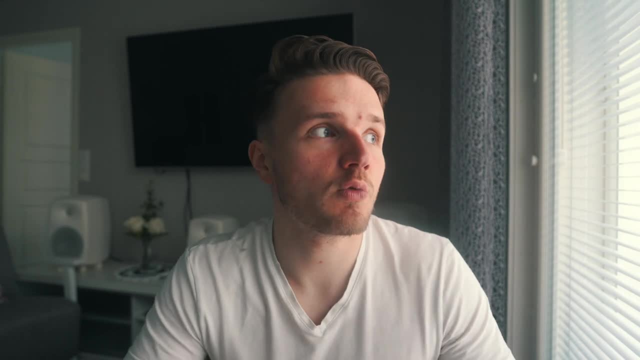 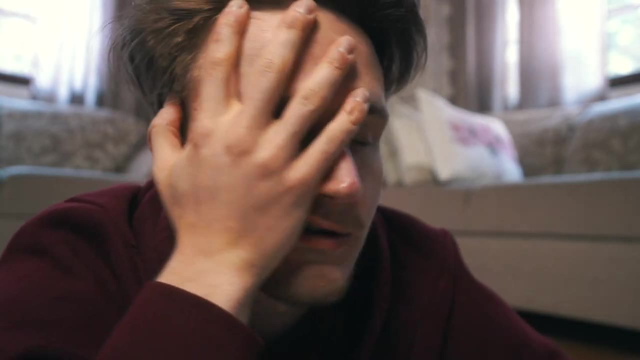 my university degree, that's. so that's what goes my mind. that is the only reason why i wasn't able to do a lot of the exercises, because i didn't want to do it when i wouldn't have any idea of whether i'm even doing it right, and so that was just quite demotivated. as when it came to the 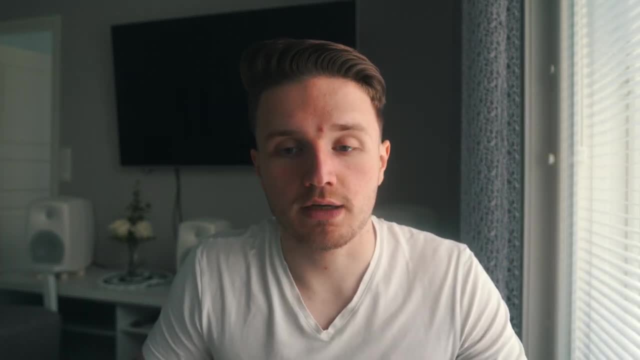 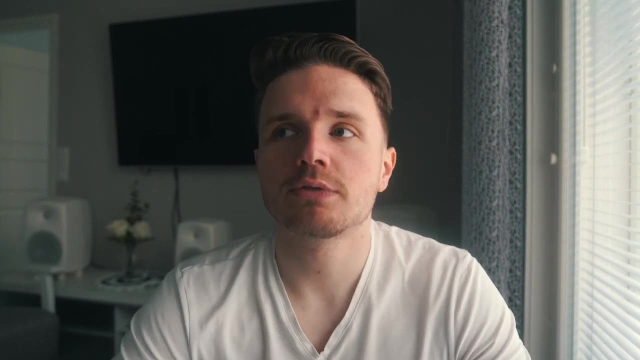 exercises. that is probably the biggest downside of the course, in my opinion, in terms of the quality of instruction and how engaging it is. it's not like the most engaging in the world, but at the same time it's better than a lot of the university professors that i had in my own. 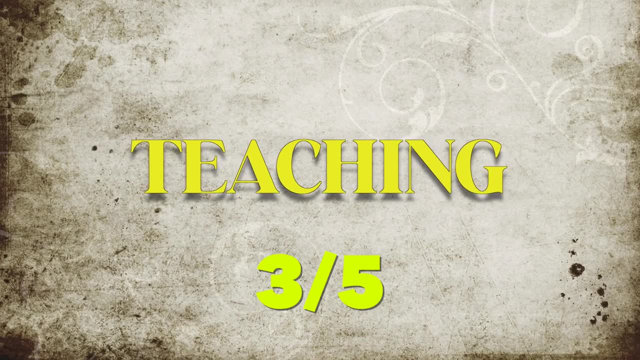 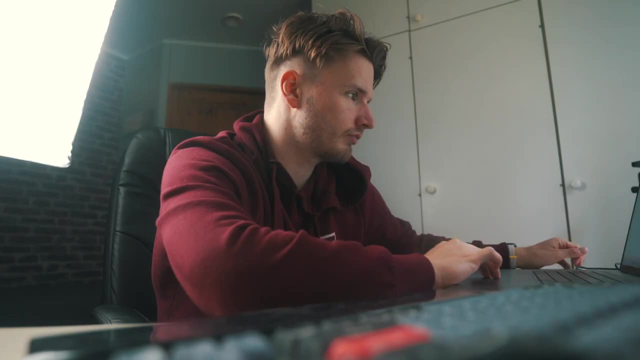 university degree, for example. i think the teaching is good. i think the textbook explains things well, but they are very mathematical explanations and, as i said before, it is a very theoretical course. you do need to spend a lot of time thinking. you probably need to read through the same thing a couple of times. 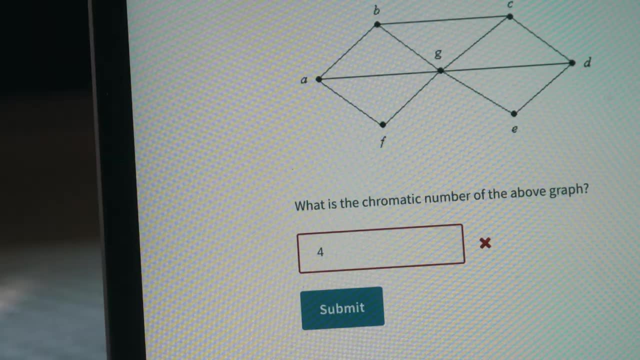 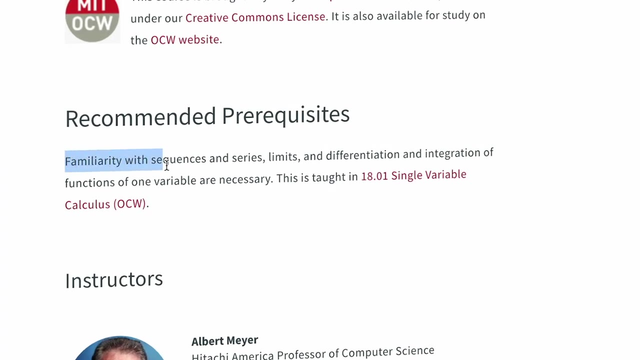 to really understand these things because they are not easy and math is not easy, so not much else i can say about that. really, you do need to have like high school level math down when you go into this. like you need to understand algebra. probably calculus is helpful because 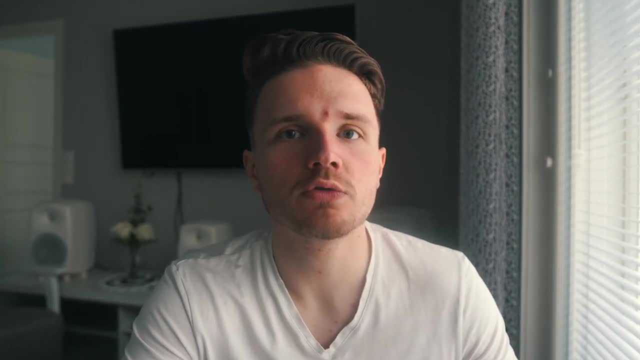 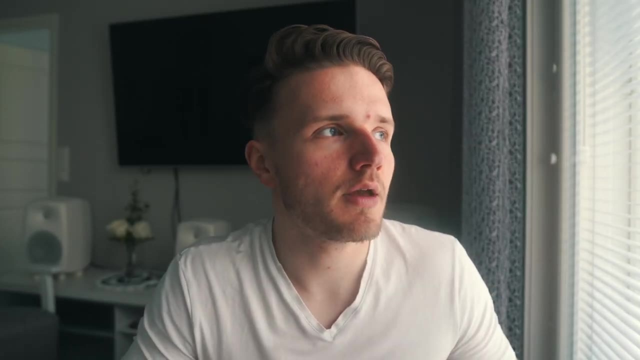 essentially this is a university level course. you can't just go into it not knowing anything about math if you don't understand the basics of algebra, but if you don't math at high school, you should have that. but beyond that i think it's reasonably approachable as far as maths go. so 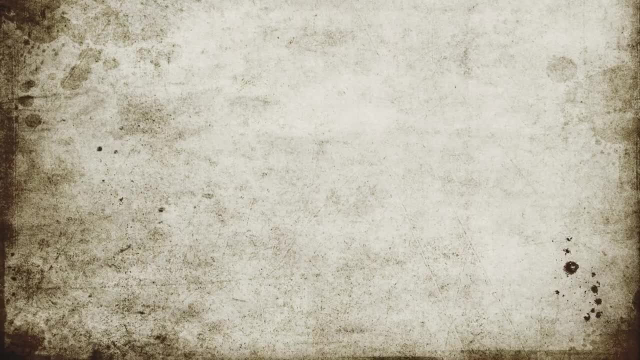 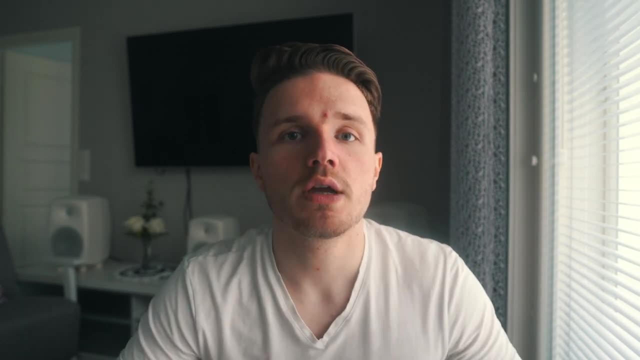 not much to complain there, and in terms of cost, it is completely free. you can do it for completely free online. in terms of comprehensiveness, well, it's very thorough. it teaches all the math that you would ever need to know in terms of computer science, i believe, with the exception of linear. 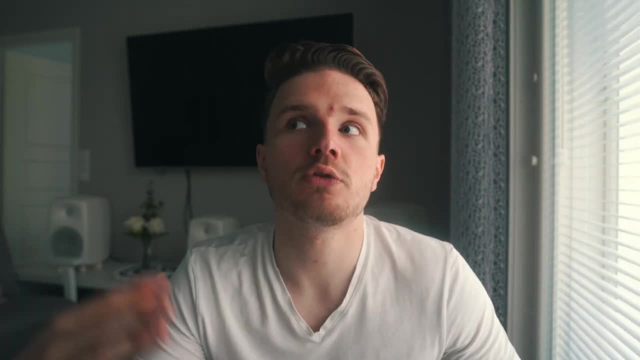 algebra. i'm not going to go into too much detail about that, but i think it's a really good course and maybe there's some like other topics of math you would still need to learn if you go into the specific areas where these are useful. for example, i'm trying to self-teach ai right now and for that 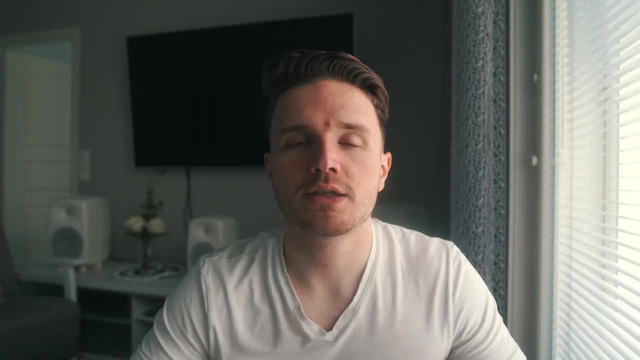 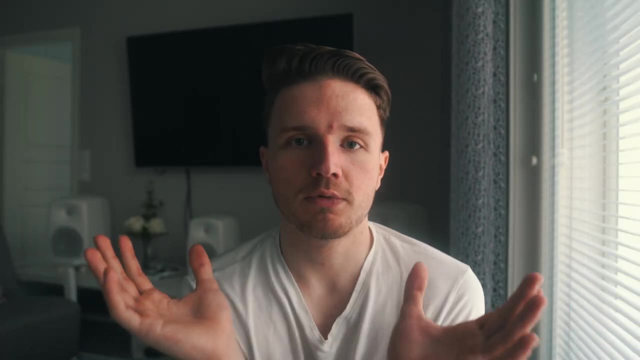 i do need to understand linear algebra or matrices and vectors, and this course doesn't go over that. so there are some areas which you would need to study separately to this, but basically most of the maths, for, like the broad areas of computer science and programming, this course teaches you. 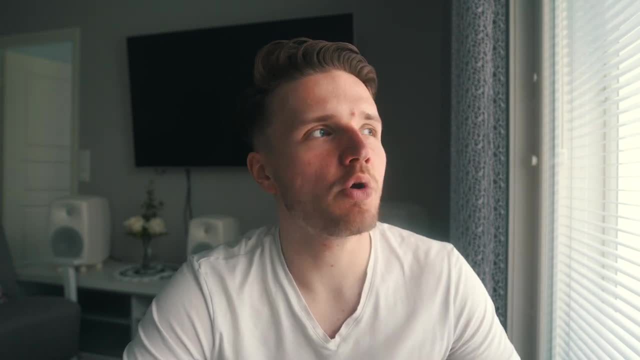 so it's very comprehensive, but this is sort of where we come to the main point that i wanted to get across here. there are a lot of people who are interested in computer science and programming. there are a lot of people who are interested in computer science and programming. this course teaches. 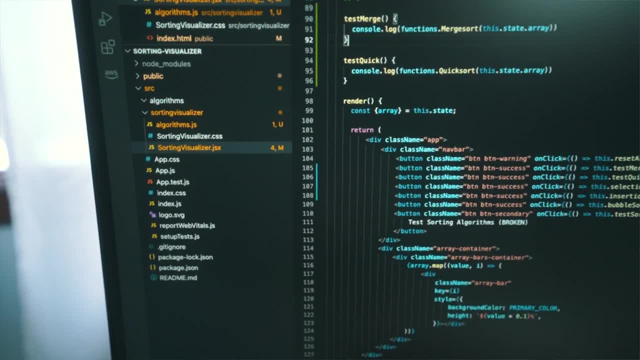 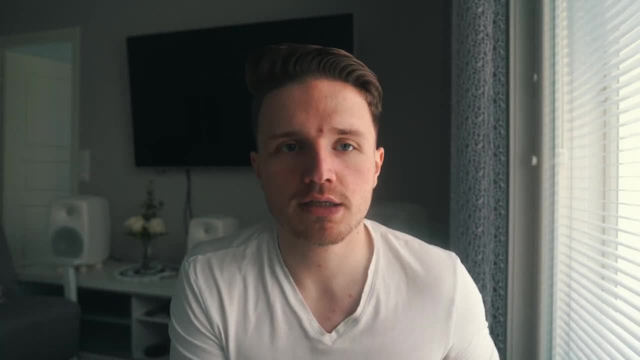 a lot of people like, for example, if you just want to learn to build websites, you just want to learn web development, you just want to become a good programmer and you don't specifically care about the theory of computer science and like all the different areas of computer science, like 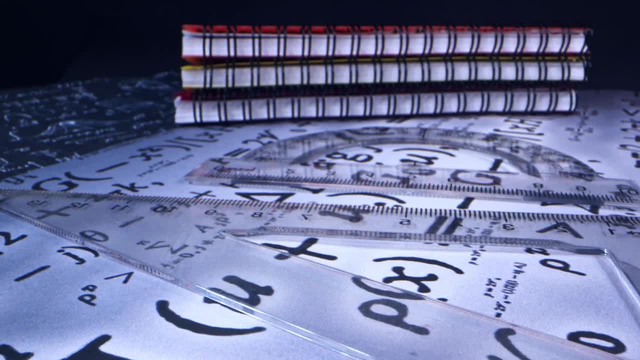 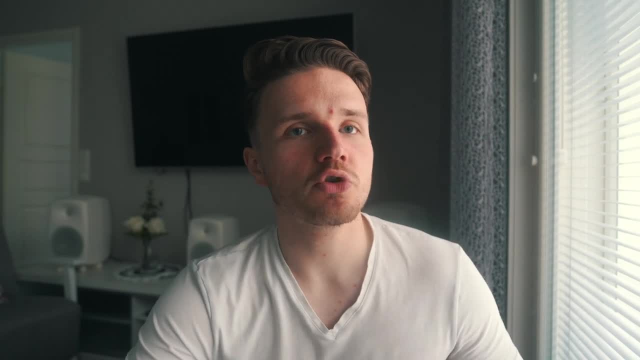 cryptography and all these different things that you won't even need as a programmer. you probably don't need to do this course. you probably don't need to learn all the things that this course teaches you. there are some areas of the course which you should absolutely understand if you. 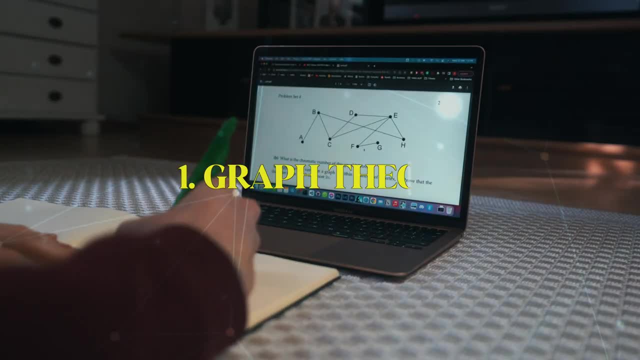 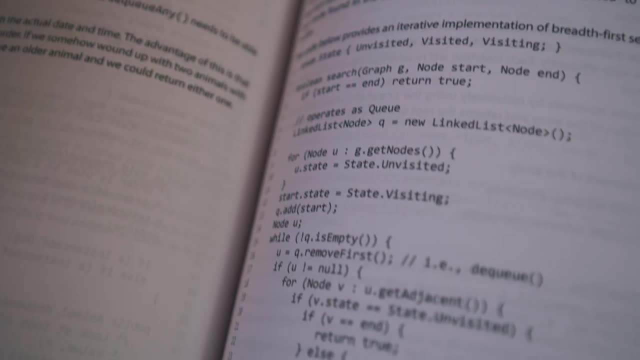 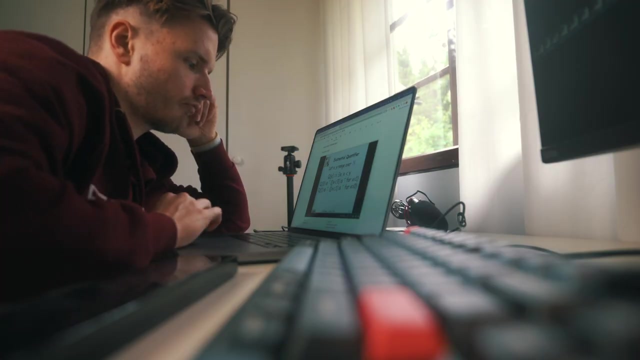 want to be a great programmer down the line, like, specifically, graph theory, especially if you want to apply for a lot of the big tech companies. they will have data structures and algorithms based interviews and a big part of data structures and algorithms in programming is graphs and to understand graphs is really helpful to understand a graph theory. you kind. 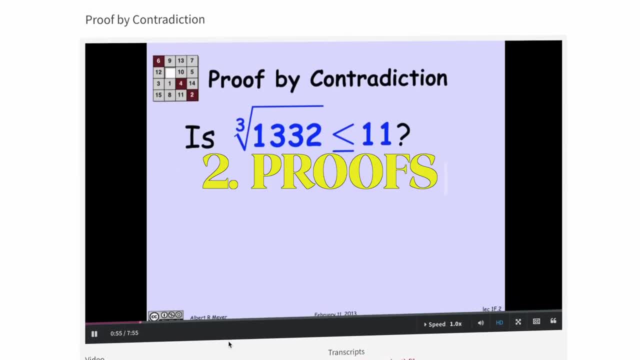 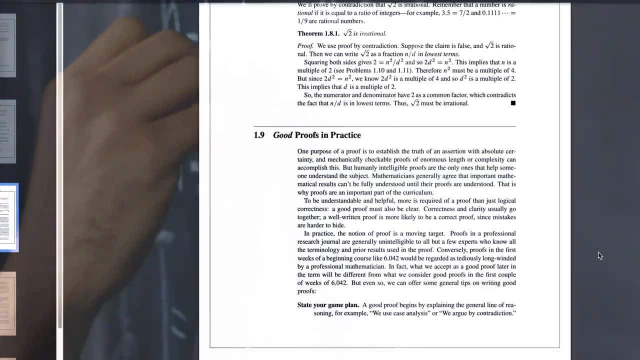 of need to understand mathematical proofs, because the way a lot of the running times of algorithms are proven are using these inductive methods, for example, that you will learn in the first part of the course. so i would say there's sort of two types of people with this. on one hand, people who really 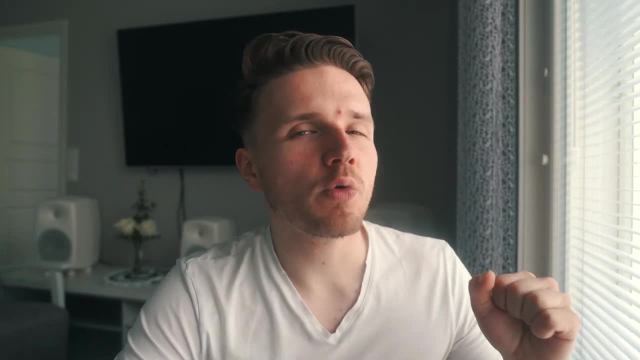 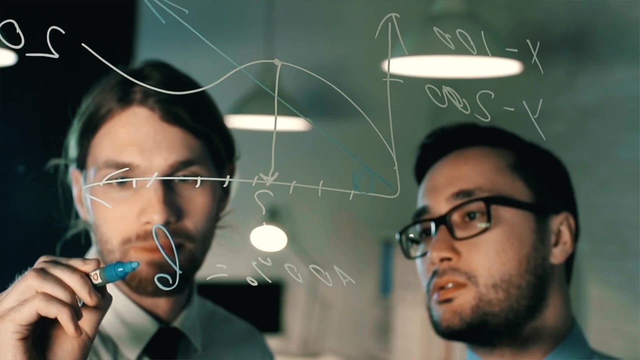 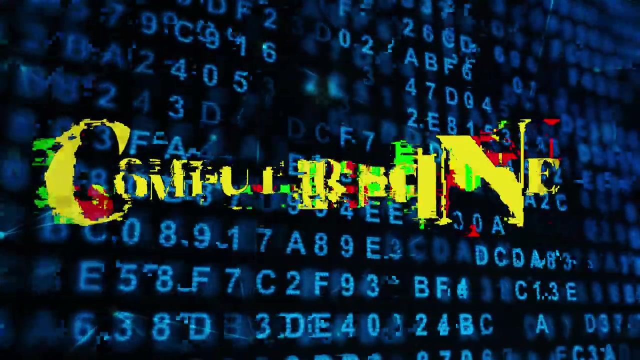 want to learn about not only programming but computer science and, specifically, if you want to apply to and get into the top top companies. for this, it's undeniable that there are some areas of the maths of computer science that you absolutely should understand, because programming, at the end of the day, is based on computer science, which itself is a subset of math. on the other hand, 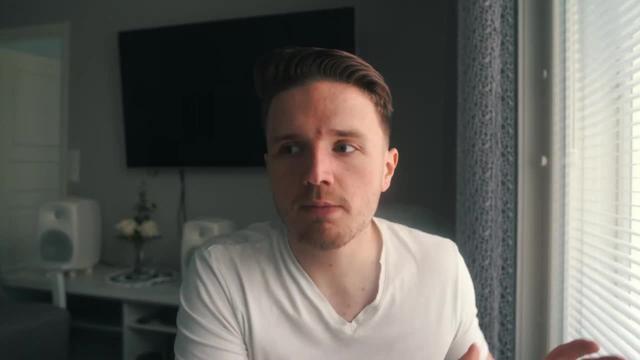 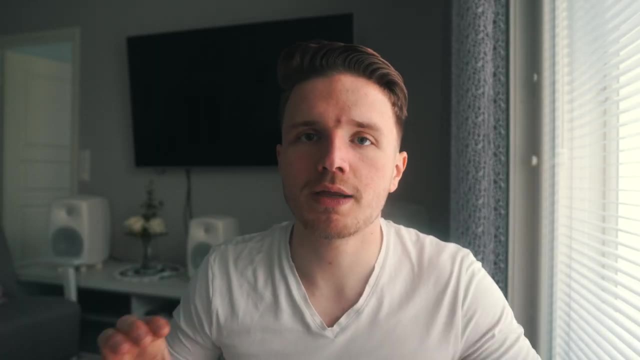 there's a lot of people who don't perhaps care about getting into the fan company, so you just want to be a programmer at like an insurance company or something like that. who knows how to you can build a really great career never even knowing any of these things. even beyond that, i 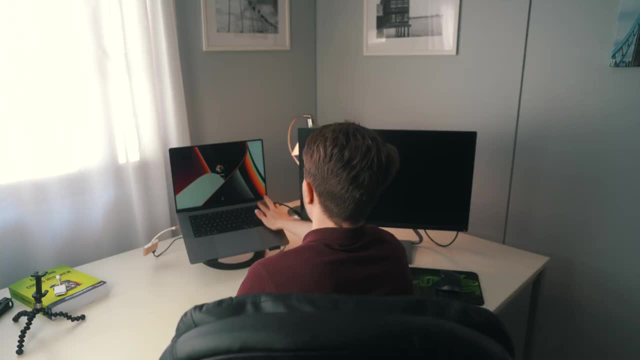 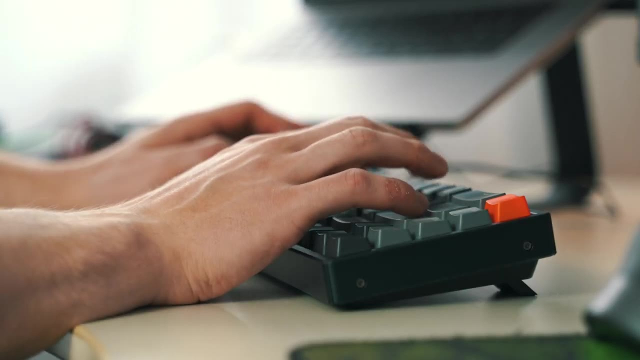 am definitely in this camp or like i want to learn more, even if some of it is going to be useful. just in case there is that 0.01 percent of cases where it's going to be helpful, it's gonna put me above some other programmer who doesn't understand some of the underlying detail. 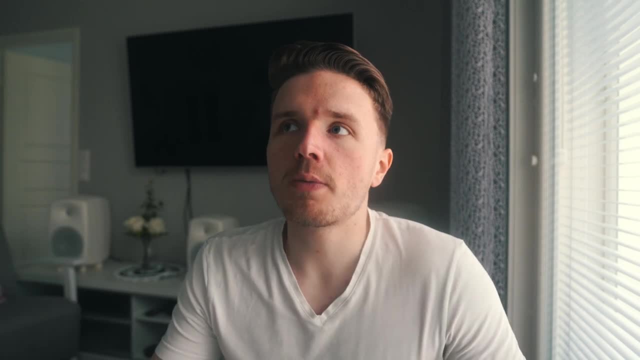 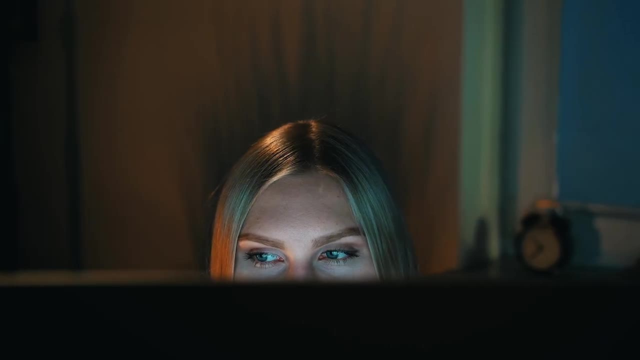 so for me, doing this course was worth it, i would say for a lot of people. actually, what you probably should do is just focus on learning to code and then, along the way, figuring out if there are any parts of math that are useful in the specific area that you're going. 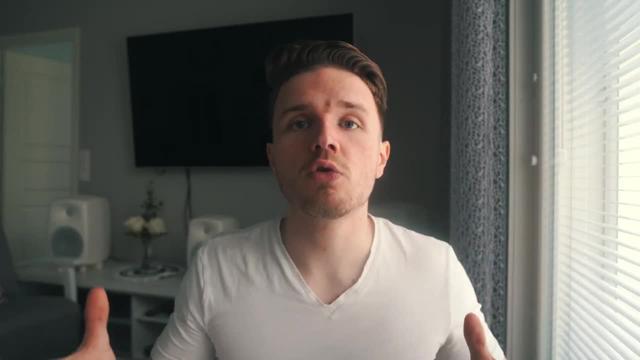 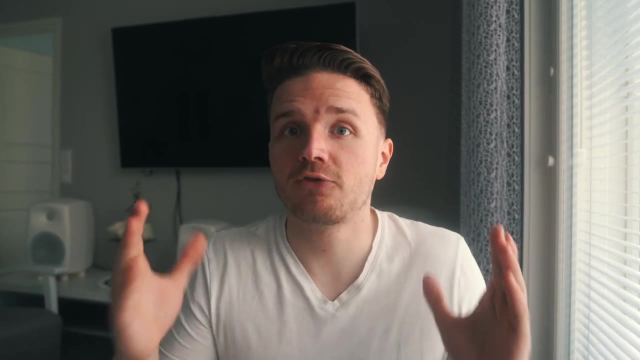 into and then just learning that. but if you do decide to do a course on maths for computer science, this is the course. this is probably the only course- at least the only course that i could find online that is free, that teaches you all of it in one place. so if you do want to learn it, then 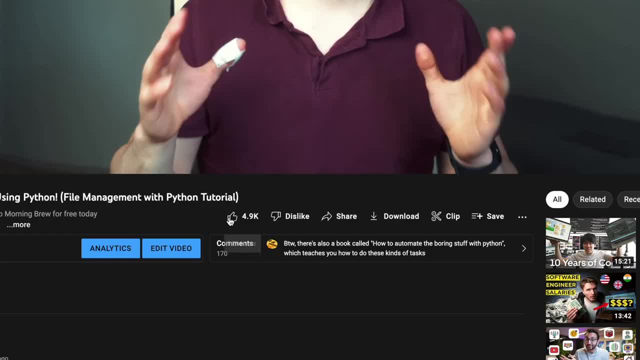 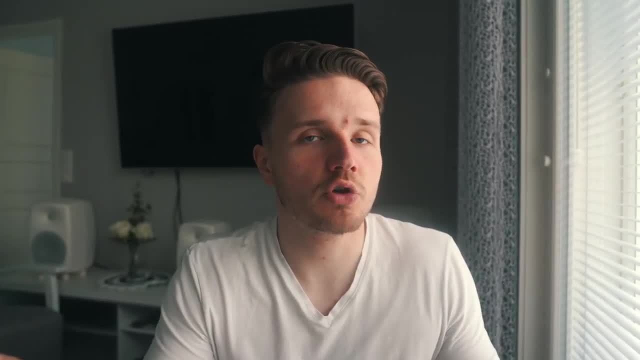 this course gets a big thumbs up. if you enjoyed this review, make sure to hit the like button down below in the description, because it shows youtube algorithm that this video was helpful to you and it will show it to more people now. if you're new to this channel, you're very welcome. my name is 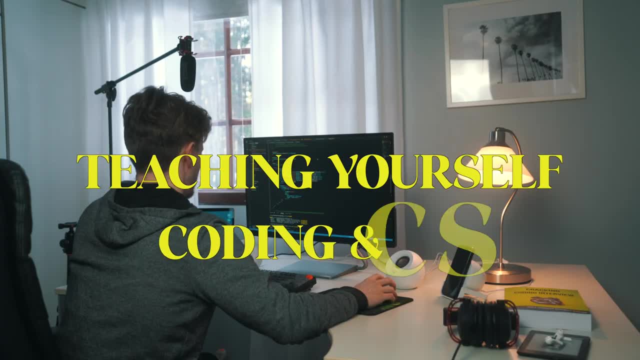 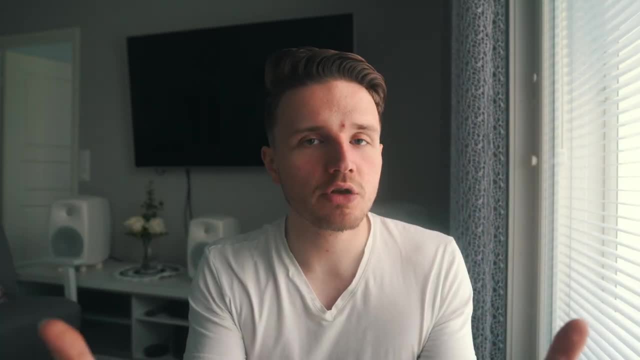 internet coder, and this channel is a place for people just like me who are teaching themselves coding and computer science. so the purpose of the channel is for me to give to you everything that i have learned along my own journey of self-teaching coding and computer science. so if that 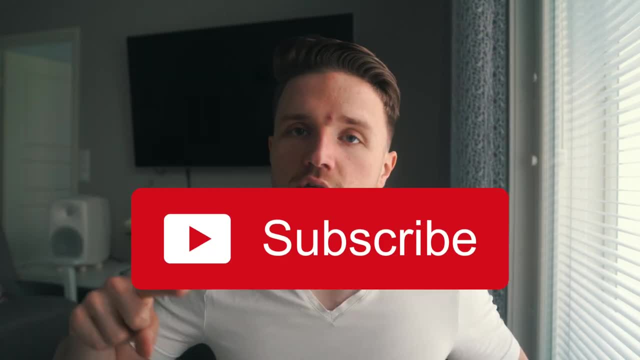 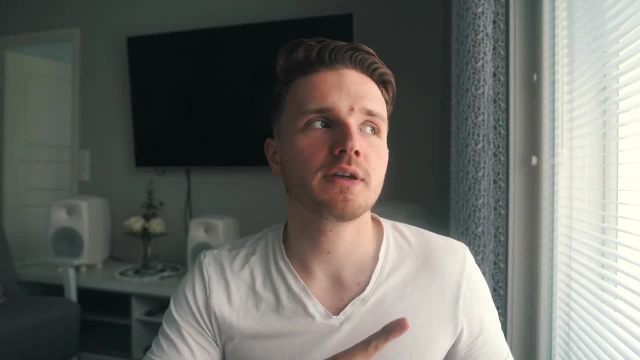 sounds interesting to you, make sure to hit the subscribe button down below so you don't miss my next video. if you want to avoid the biggest mistakes that most people make when they're learning to code, i highly recommend you watch this video. until the end of the video and i'll see you.